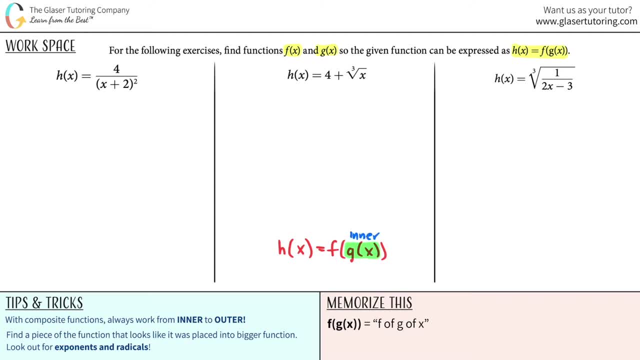 the inner function and that is meshed inside of the f of x function, that's the outer function. When you're trying to, you know, make your function so that you get your composite functions, it's always easiest to work from inner to outer. Okay now, since we have to, you know, 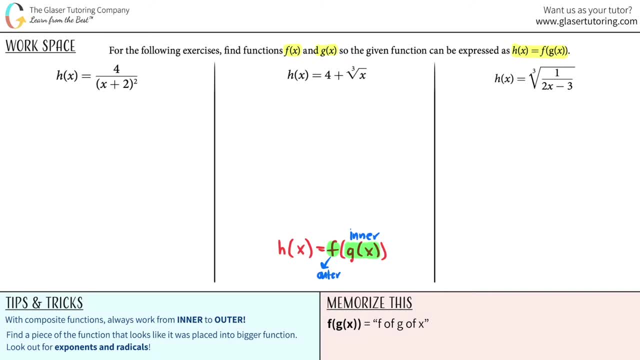 get the pieces of the puzzle. here is a quick tip. You're going to find the piece of the function that looks like it was placed into a bigger function. You're going to look out for exponents and radicals. Okay, so for the first one, I have to find out what f of x was and what g of x was Always work. 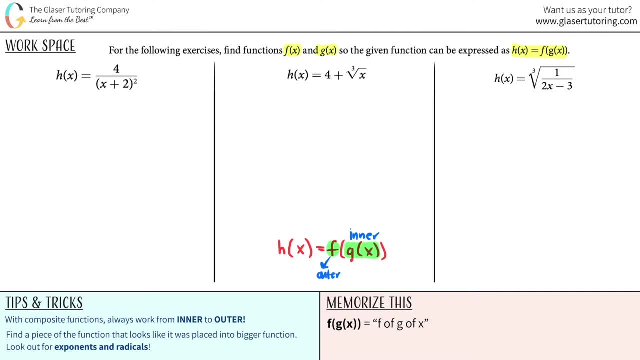 from inner to outer and make sure that you can decipher what is inside keyword inside something else. So for here it was 4 divided by x plus 2 squared. Hmm, it looks like this: x plus 2 is surrounded by these parentheses. race of the second. 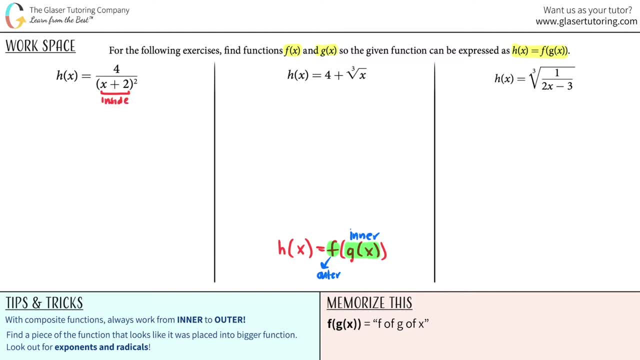 Hmm, it looks like this is inside keyword, this race of the second. Oh, inside inner tomato tomato. What do you think the inner function was? And the inner function here they want g of x. The inner function is x plus two. 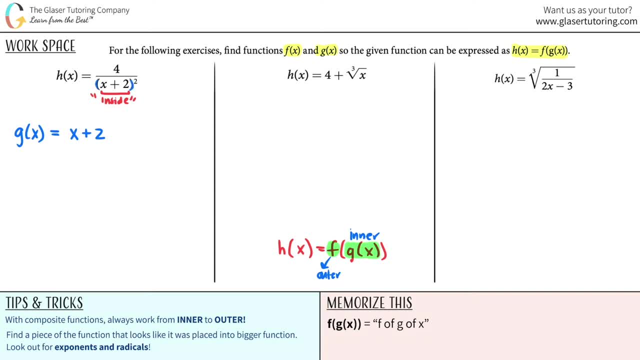 because that's trapped Stuff, that is trapped between parentheses or square roots or cubed roots. that's always going to be your inner function. That's the hardest part. Now comes the easy part For the outer function, which they wanted as f of x. 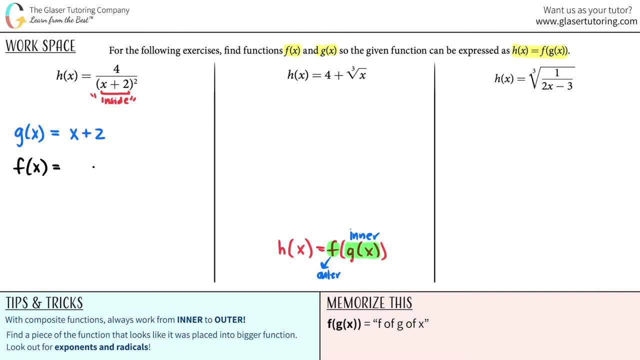 all you gotta do is just rewrite the main function. So I'm just gonna do that for you guys here And in your mind. I mean, you don't really have to do this on paper, but maybe, starting off, you might want to. 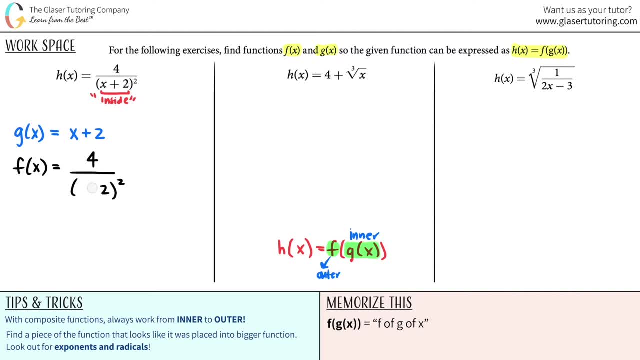 But what you're doing is you're going to erase everything that you stated that was the inner function. So that's why I erased everything in here And you just replace it as an x or the letter that you know they give you. 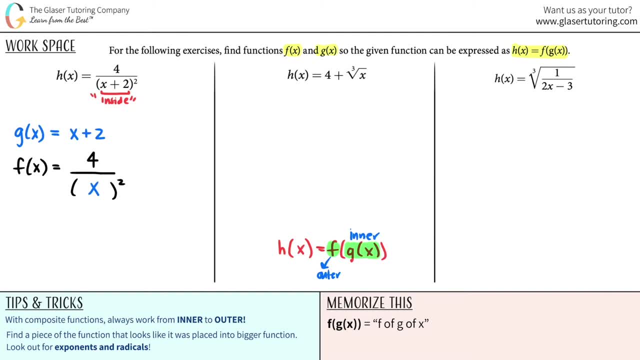 So if they give you like a t, you gotta put a t down here. The letters have to match, And now all you gotta do is just clean it up. So f of x was four over x squared. I don't need parentheses if I'm just gonna say x. 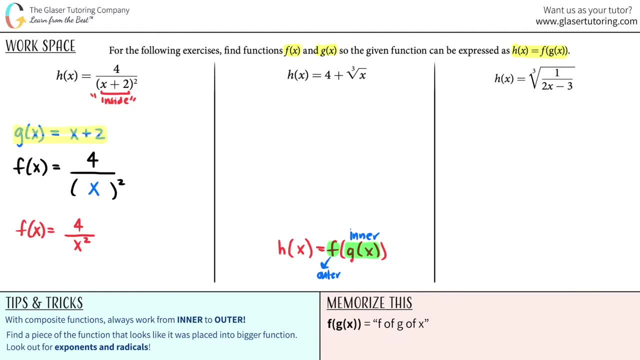 And those are your two functions. So the inside function was g of x, x plus two, And the outer function was four divided by x squared, And that's it Pretty easy, right? So always think of what is inside or trapped inside something. 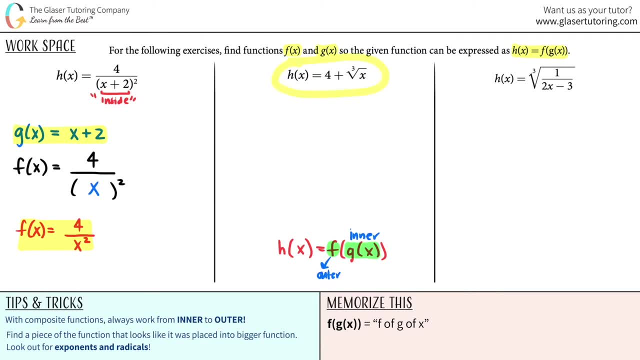 Okay, so now moving on to the second one: h of x equals four plus the cubed root of x. Hmm, I don't really see anything really trapped or inside of parentheses, So that's not really gonna help us. However, I see two distinct entities. 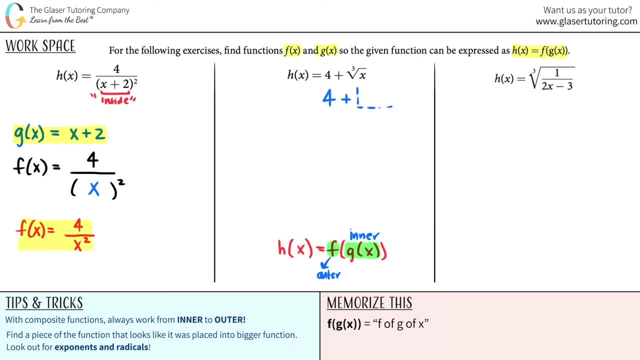 I have a four plus something else that has a variable in it, right An x. Oh, maybe I can, you know, turn that into an outer function. I can say that this whole thing was the outer function And I can say that this whole thing. 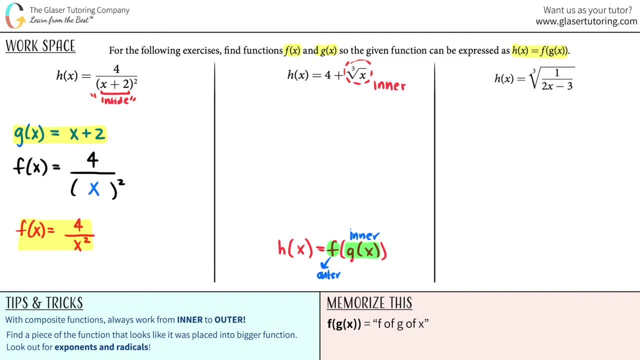 was the outer function And I can say that this whole thing was the outer function And I can say that this whole thing was the inner function that was placed inside of the bigger function. So let's see: g of x would equal. I'm going to say that the inner function here 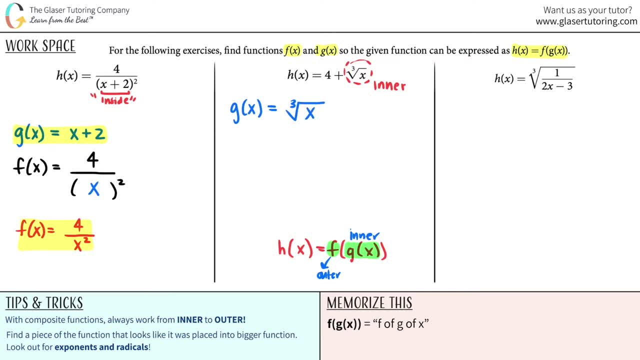 is the cubed root of x. Now for the outer function. all you gotta do is just mentally- I'm gonna write it down- but mentally erase what you said was the g of x and just represent it as just an x value. 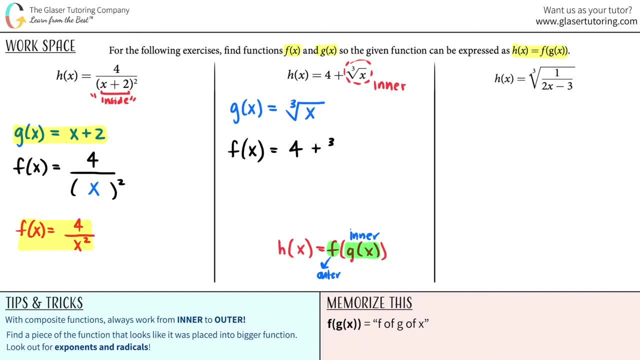 So here it was four plus the cubed root of x. but erase what you just said was your inner function and put an x there. There you go, Clean it up. I mean this is pretty nice and standard: Four plus x. 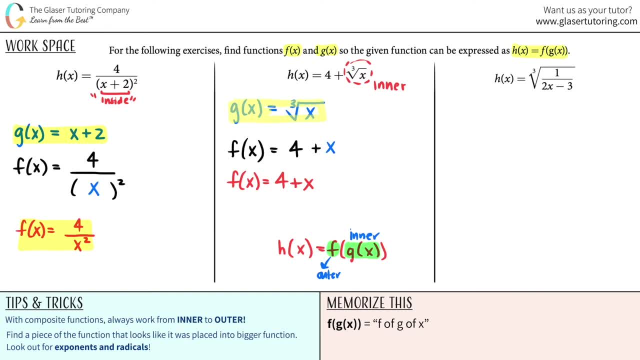 And those are your two functions. So sometimes you'll use your inside notation and what we did when we did this one, but you don't have to do that. So you don't have to do that. So you don't have to do that. 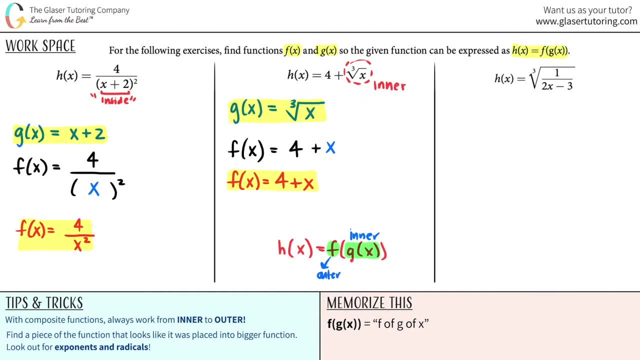 But sometimes you could split up the function in two different things. Okay, let's go to the last but not least. Let's see: Okay, this one is just the cubed root of one over two x minus three. Hmm, Well, there's nothing after this, right? 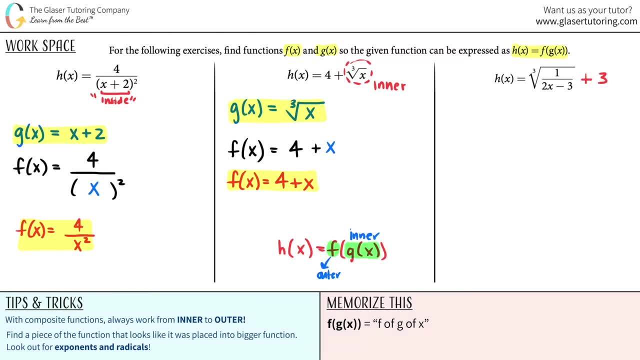 It's not like plus two or plus three, So I can't make this whole thing being x, but is there anything trapped inside of something else? It looks like this whole fraction, right, The one divided by the two x minus three is inside the cubed root. 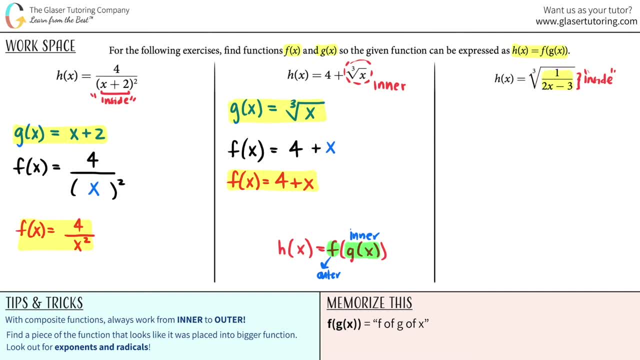 You see how this whole thing is trapped underneath the cubed root. So if that's inside, that's the inner function. So g of x would be one divided by two x minus three. Now all we gotta do is just make the outer function. 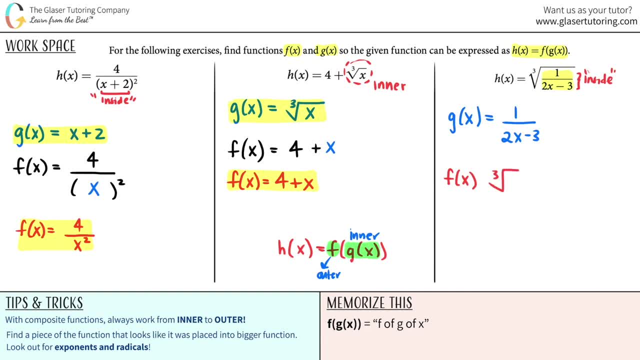 So remember, just rewrite it, or mentally rewrite it and then just get rid of what you said was the inner function and just label it as x. So, okay, all this was the inner function, I get rid of it and it's just an x. 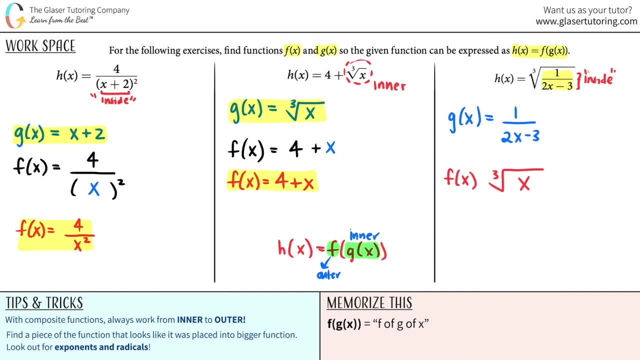 And that's that I mean. I can't really clean this up, right Cause it's all the same. So I'll just make it a little more pretty and I'll put an equal sign here. Let me just make it the same color. 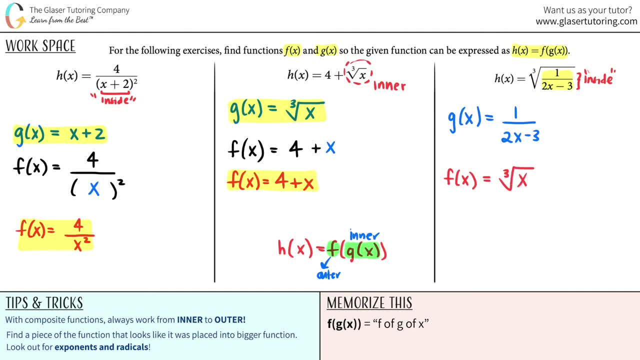 Okay, so this is equal to the cubed root of x, and that's it. So here are your two functions. Once you guys get more practice with this, I mean you guys are gonna be great, I promise you. But practice, practice, practice, especially for math.